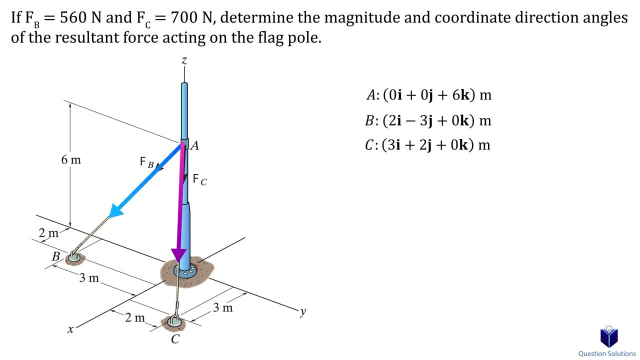 So it's just a vector that starts from where the force starts and then ends where the force ends. first, look at force FB. Notice how force FB starts at A and ends at point B. So to find the position vector we just subtract the position of A from the position of B, So we're. 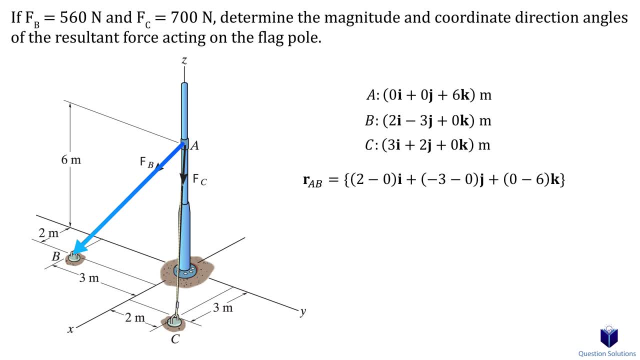 just subtracting each component of A from B. Just a tip: when we look at the way we wrote RAB, B is the last letter. So when we subtract, we actually write B first and A comes second. so we're subtracting A from B. If you keep that in mind, you won't mix. 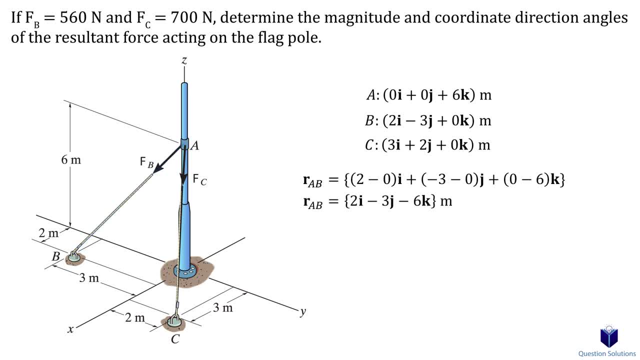 them up. Let's simplify. Let's do the same for force FC. So it starts at A and ends at C, which means we subtract the position of A from C. Now we will find the magnitude of each of these position vectors. We do that by taking each term, squaring it, adding it. 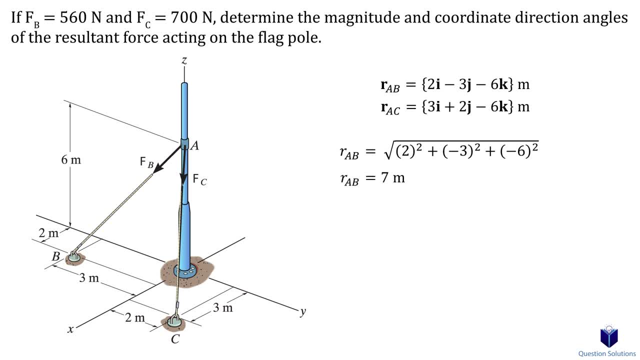 all together and then taking the square root of it. Next, RAC. By the way, these magnitudes we found is the distance from points A to B and A to C, In other words, the length of each rope. Now that we have the magnitude we need to find, 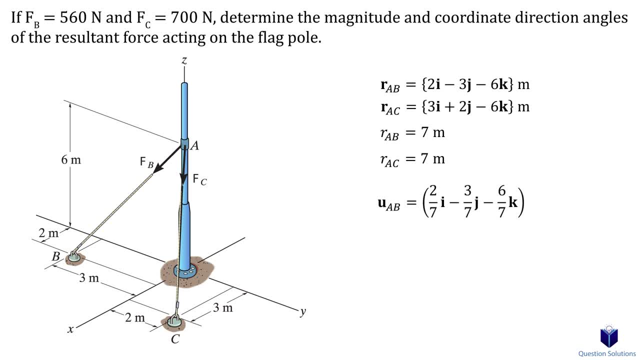 the unit vector. We do that by taking each term in our position vector and dividing it by the magnitude. So the last step in expressing our force in Cartesian form is to multiply it by the unit vector. So for force FB, we're just multiplying each term in the unit vector by 560 Newtons. Let's. 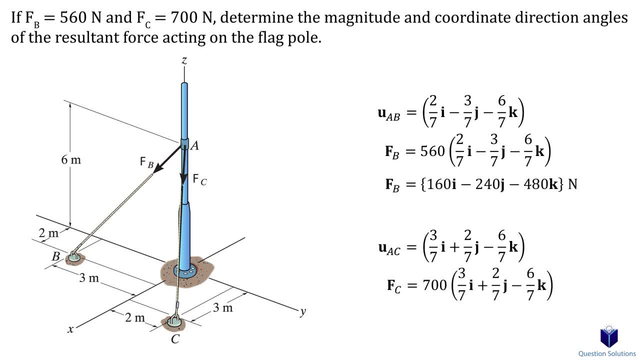 simplify. Next we have force FC. So again, all we do is multiply the magnitude of the force by the unit vector. So now that we have our forces expressed in Cartesian form, we can add them together to get the resultant force. We just add I components to I components. 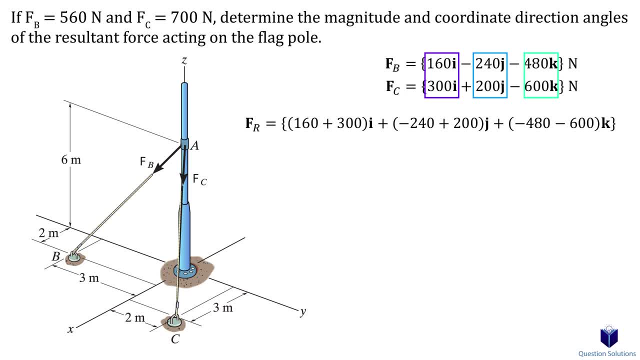 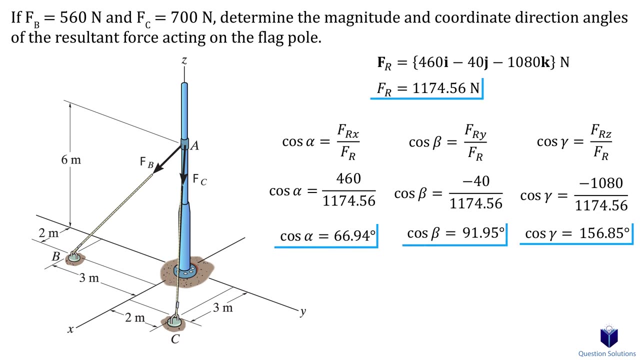 J components to J components and K components to K components. The magnitude of this force can be found the same way we did before To find the coordinate direction angles. we can use these equations. If we take the inverse of cosine, we get our angles. Those are our. 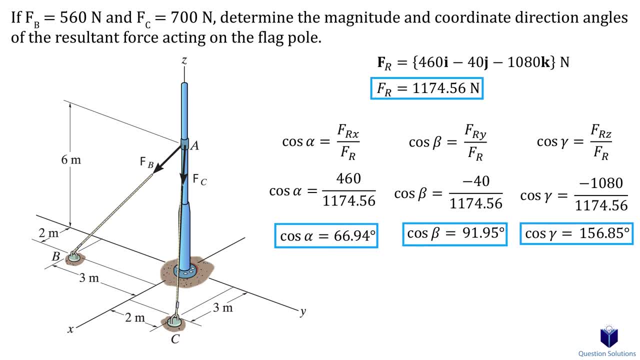 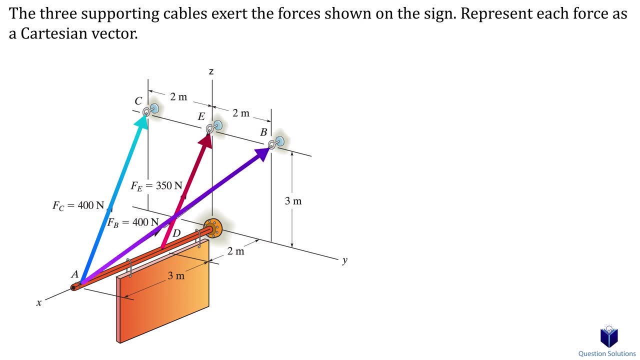 answers. If these equations are unfamiliar to you, please check the description for the previous video about the addition of Cartesian vectors, where I discussed them in detail. Let's take a look at this question, where we need to express each force in the ropes in Cartesian form. So the first step is to write down the locations of points A, B, C, D and. 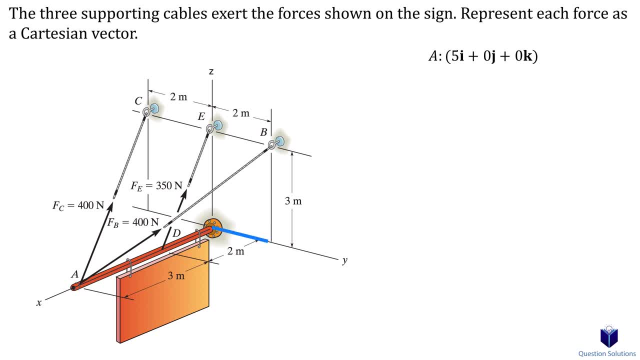 E, First point A, Next point B, First point C, Next point D, Next point E, Next point C, Next point B, Now point C, Point D is next And lastly we have point E. Now we have three cables. 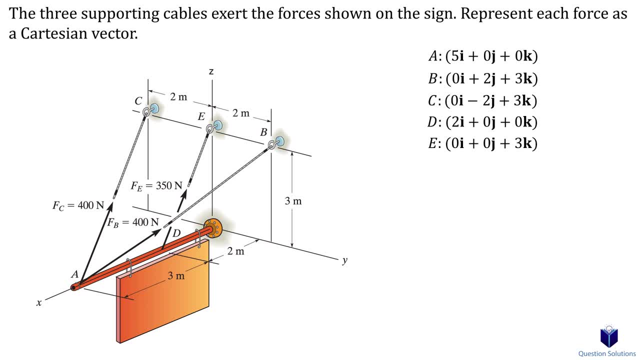 so we need three position vectors. The first will be for force FB, which goes from A to B. Next we got force FC, which goes from A to C. Lastly, we have force FE, which goes from D to E. The next step is to calculate the magnitude of each of the position vectors. 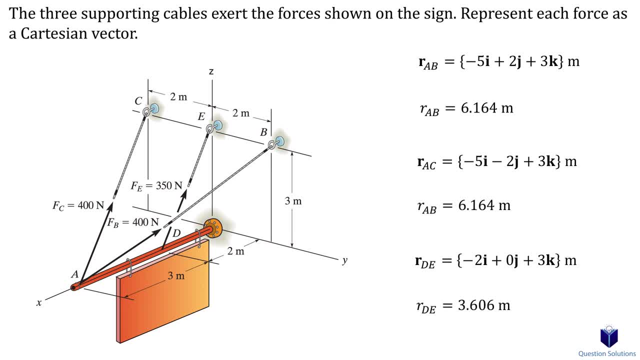 Now that we have the magnitude, we can find the unit vectors. So remember, all we do is divide each term in the position vector by the magnitude. The last step is to multiply the force by the unit vector. First, force, FB- Let's simplify. Next force, FC. And lastly, 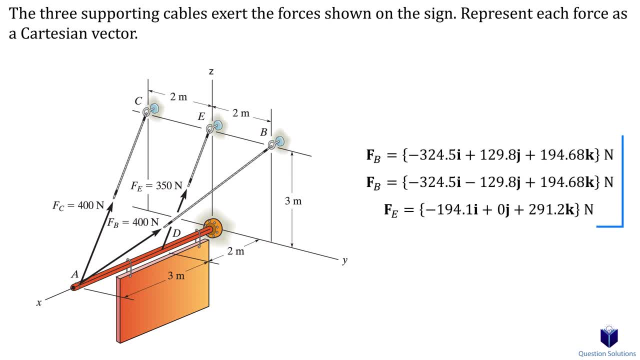 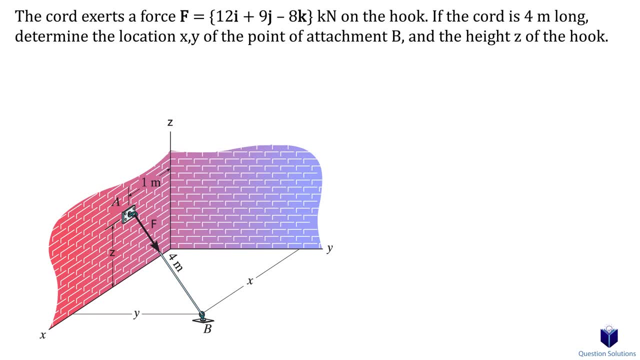 we have force FE. Those are our answers. Let's take a look at one last example, where we have a force already given to us in Cartesian form and we need to find the location of point B. So first let's write down the locations of points A and B, So when we don't know the 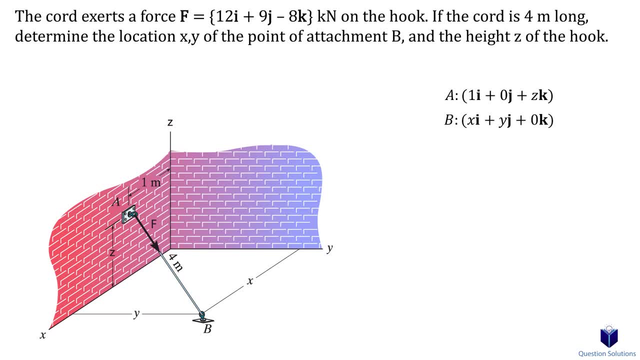 value. we will just use the X, Y and Z letters to represent the locations. Now we will write a position vector from A to B. Let's simplify. Notice that we're given the length of the rope in the question, or in other words the magnitude, So the unit vector would be each. 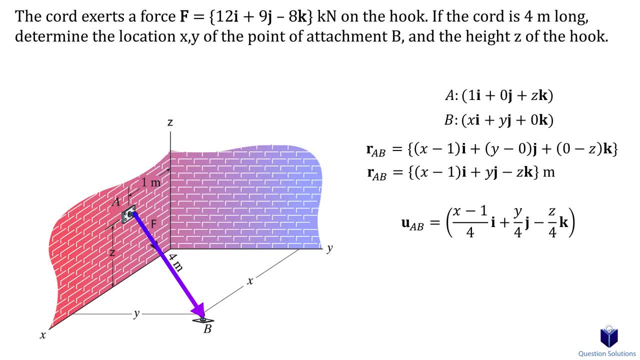 term in the position vector divided by the magnitude. Now let's look at the force given to us in Cartesian form. We can find the magnitude of this force using our usual method. So now we know that a force in Cartesian form is simply the magnitude of force times the unit vector And we are already given the Cartesian